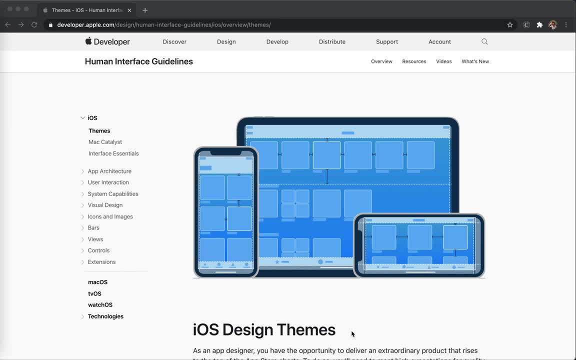 Hey guys, how's everything going? This is Jay Sir. On my channel I've already started a bunch of video series like the LeetCode one, the Weekend Channel Contest, LeetCode one. another one is CSS one and JavaScriptinfo one interview. another one is CSSinfo one and another one is CSSinfo one and another one is CSSinfo one. 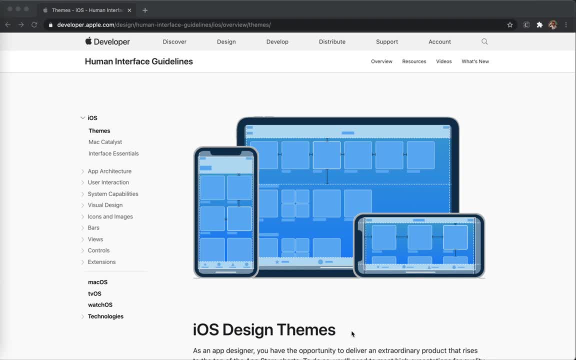 BFEdev questions. So this video is about a new series. It's about the human interface guidelines from the Apple. The reason for this one is that I recently found Apple's webpages of very super cool examples to learn things from. No matter how cool our technologies are, we must create them. 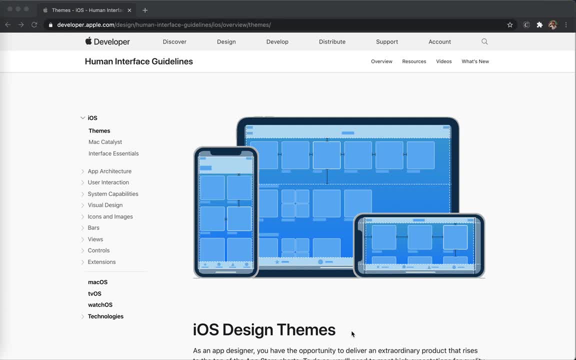 We must create beautiful products, right? So about the beautifulness that Apple is the king of the beautifulness. So, even though we are creating websites, I think that we'd better- how should I put it? We should create as closer to the native apps as possible, right? 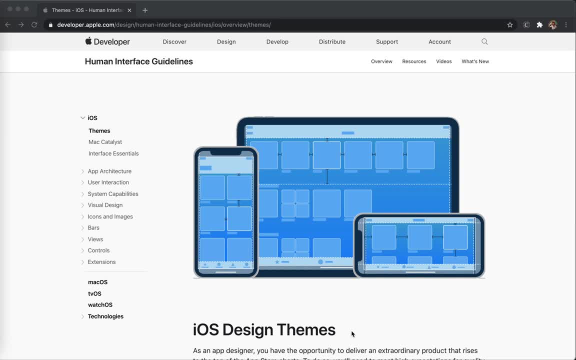 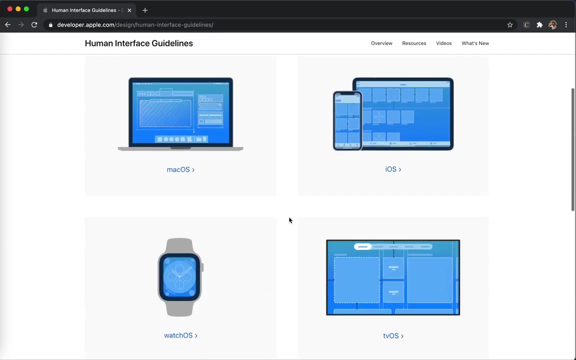 Because users are using the native apps, the operating systems. They're using the system UI every day, so they're used to it and it's better we keep consistent with that. So in this video, in this series of videos, I'm going to cover the human interface guidelines from the Apple. It's public, so if you're interested, I definitely encourage you to read through it. though I don't have any native development experience, though I've created some example apps. 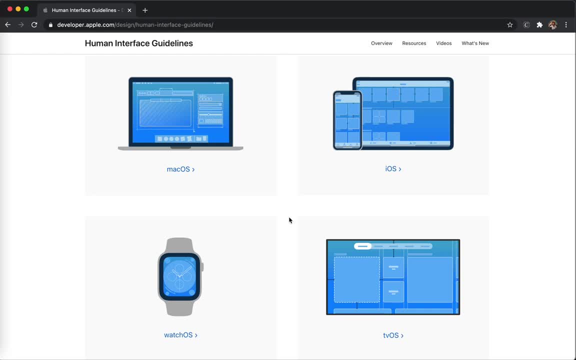 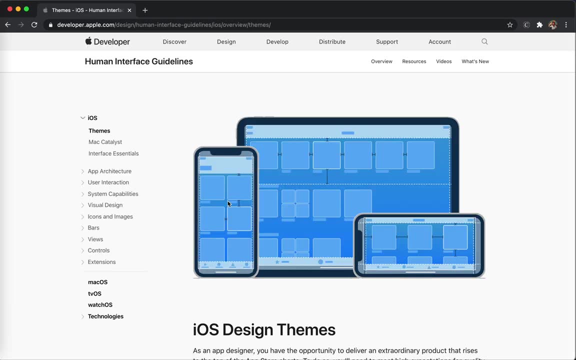 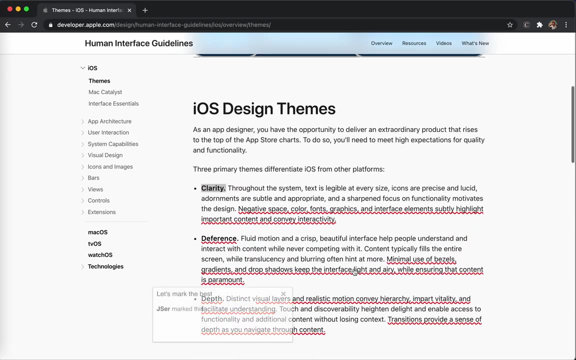 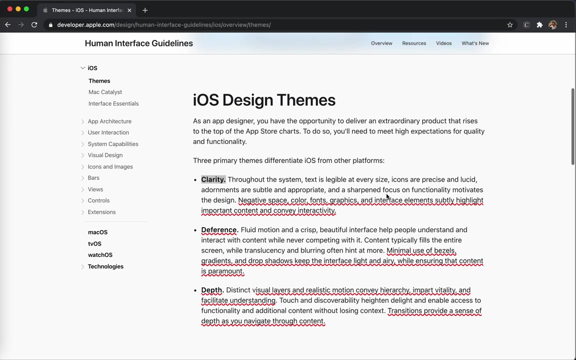 Anyway, let's first start with the iOS one. So in this video it only covers the themes and design principles. It's a little vague, actually Not that easy to understand. Let's begin. So in iOS design there are three themes. 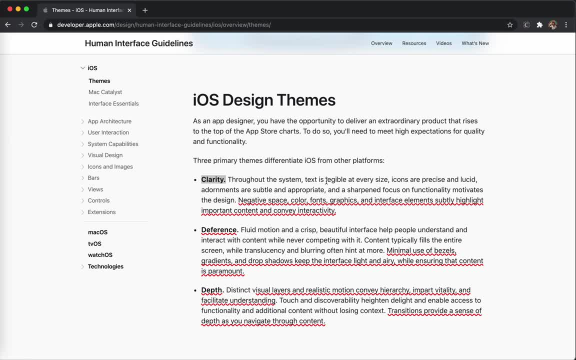 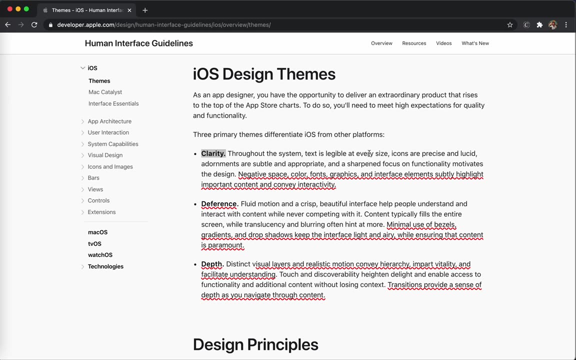 we need to pay attention to, Or how should I say? these are three metrics of how to judge if an app is well-designed or not. The first one is clarity. So yeah, and throughout the system, text is legible at every size. 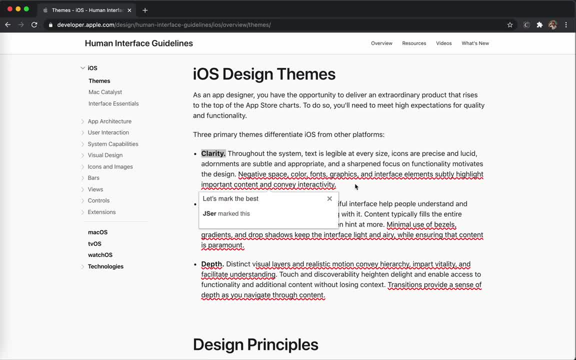 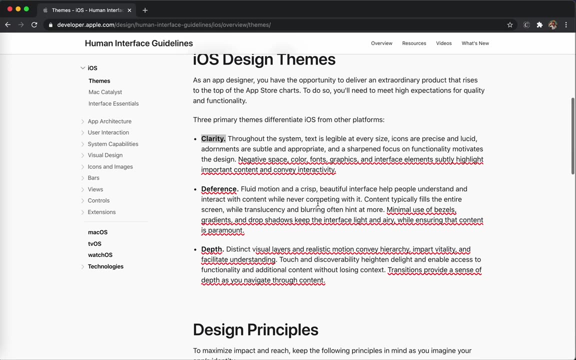 The icons are precise and lucid. We should use the right negative space font colors. Yeah, so to subtly highlight important content and convey interactivity. So it made it clear. yeah, Another one is difference, Fluid motion and crisp, beautiful interface. 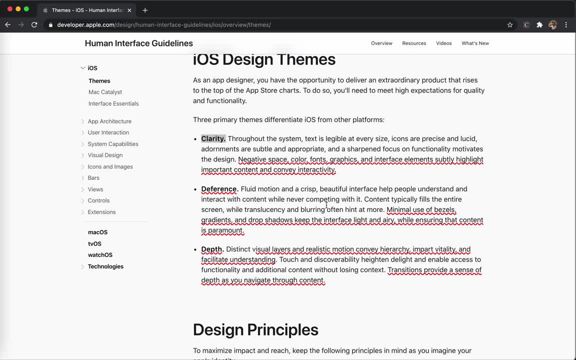 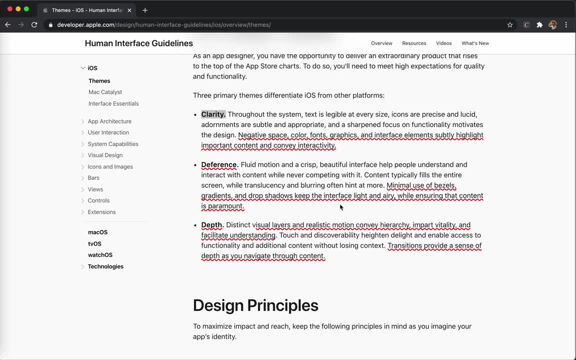 help people understand, interact with the content, while never competing with it. This is a little, I don't know what it is, So minimum use of Bezos gradient when shooting. the content is paramount. So things must be clear And we have shoot. 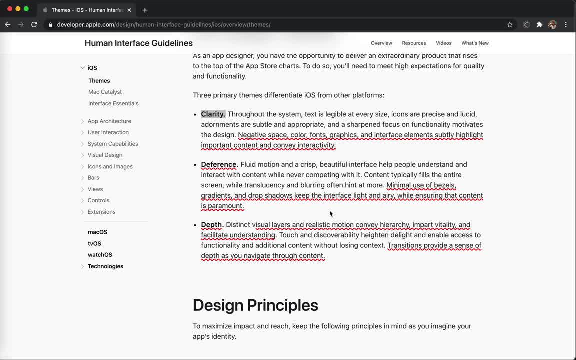 And And. the controls should be- how should I say? visually, not visually? yeah, visually differentiated, So users could know where to tap right, where to interact. Difference means this: where to interact if I want to do something. 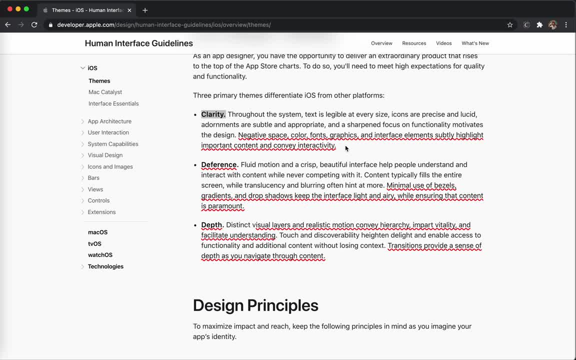 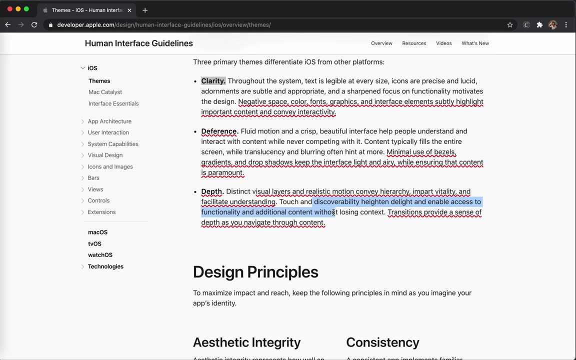 But clarity means this is interactable, This could be clickable And this means a user should instantly know where to click. OK, depth Depth actually means the transition. right, If you change the screen, like going to another screen, you could go back right. 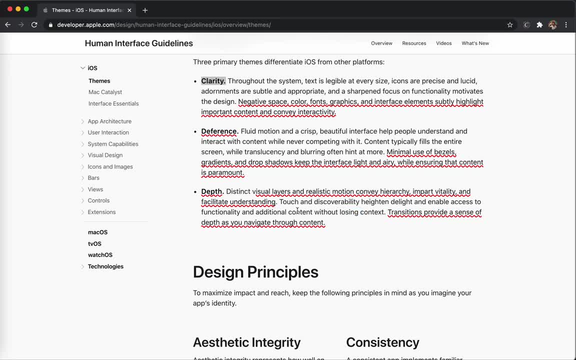 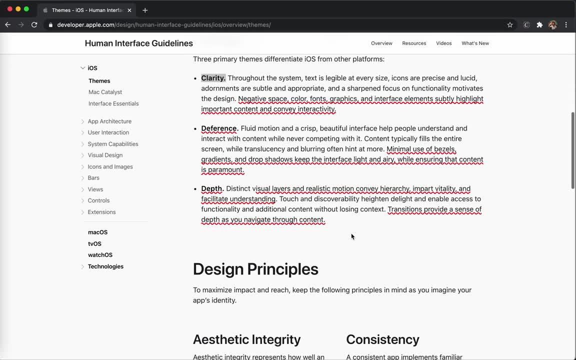 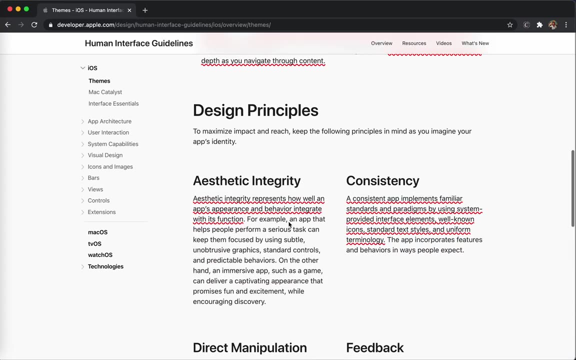 So that kind of context is very important. with the depth, It's the depth of your app. So clear difference depth- Wow, that's pretty interesting. OK, so the next one is design principles. There are some the words actually is the first time. 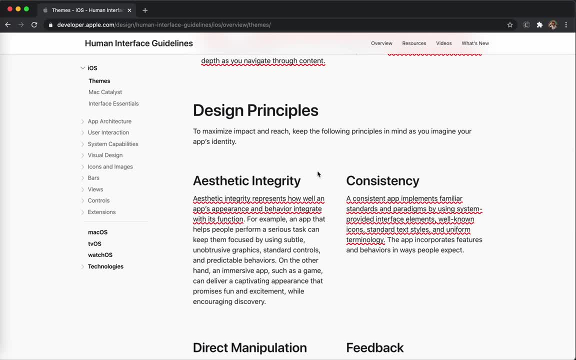 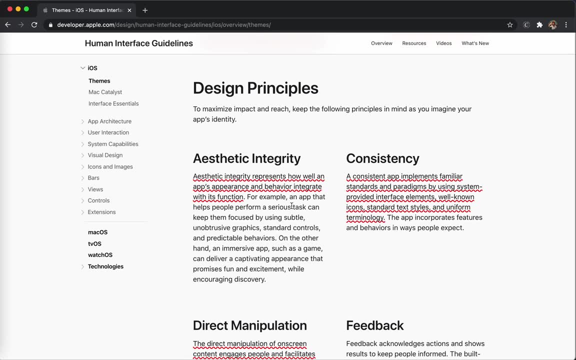 I've seen it. This is aesthetic aesthetic. OK, aesthetic integrity means how well an app's experience and behavior integrate with its function. Yeah, it's well designed, right. Detailed to the font. detailed to the color, right. Here is an example. 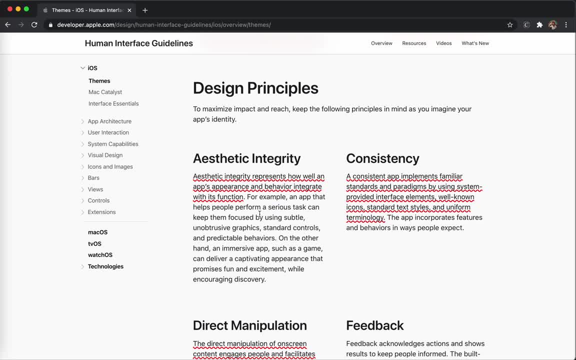 If you're creating Creating like a serious task app to keep them focused, then you should use the subtle, unobtrusive graphics, standard controls, predictable behaviors- not so fancy. If you're creating a game, you should be as fancy as possible. 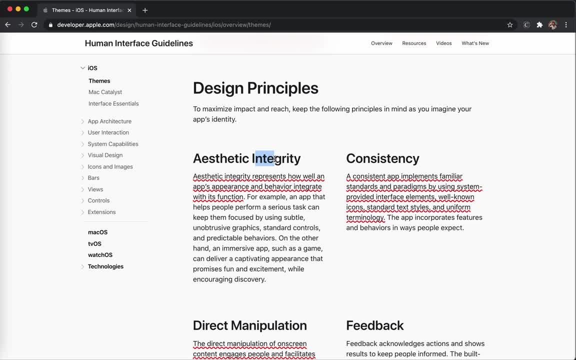 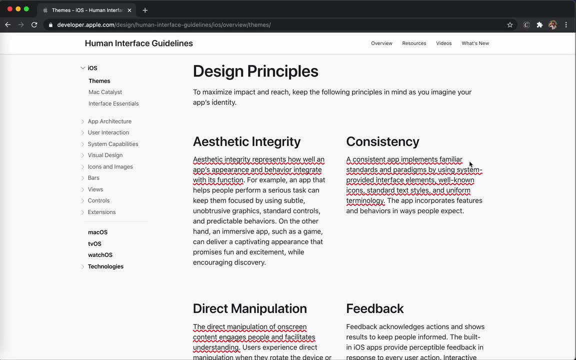 So this is aesthetic integrity. It means function should comply with the design. should comply with the function. OK. consistency OK. should be familiar and should convey with the familiar standards and paradigms Using a system providing interface elements, well-known icons. 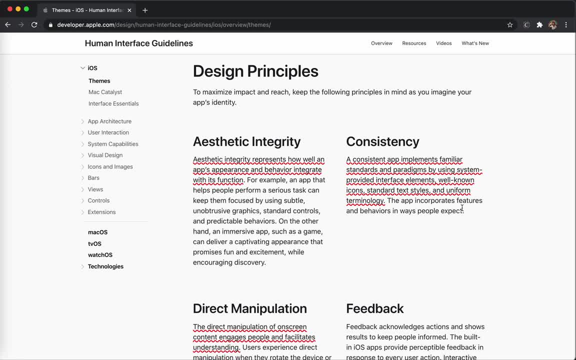 Yeah, this is what I'm talking about. Even if we're creating websites, it should be consistent with the system UI as close as we can So people don't get confused. right? If you're using an icon, you know that three dots means a menu or they have a menu. 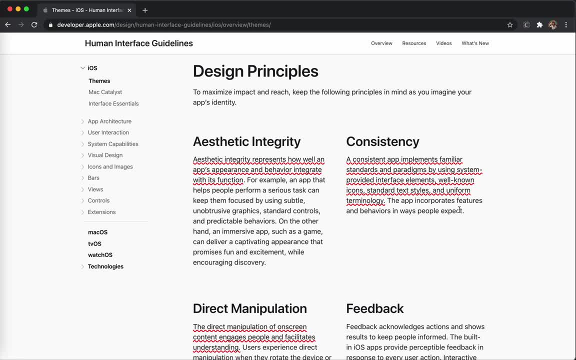 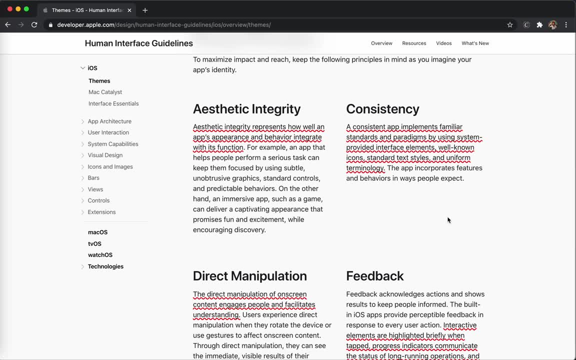 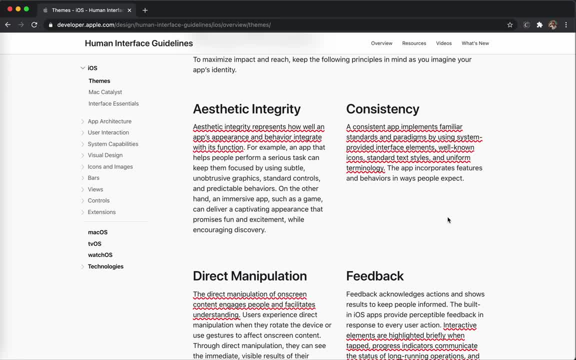 and then tap the close button and it will slide out to the right. And because users are used to that by interacting with so many native apps to us, the web application creators, we see this as a little bit of a challenge- should also try to mimic that behavior. okay, okay, so this is style from a video. 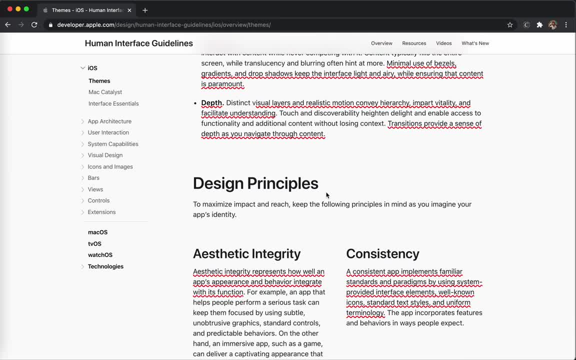 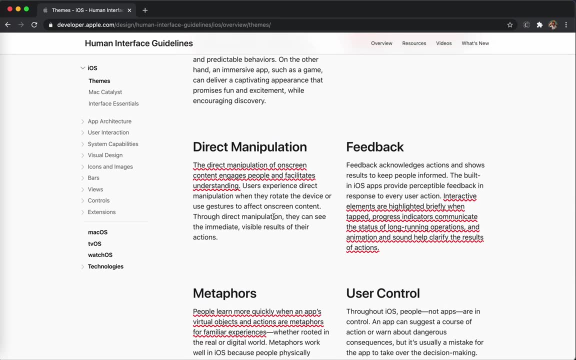 I'm going to read through the interface, human interface guidelines and pointing out as the perspective of web front and developer. okay, next one: direct manipulation. the direct manipulation of on-screen content. engage people and facilities. understanding direct manipulation. what does it mean? I don't know. user experience directive: manipulation when they rotate device or 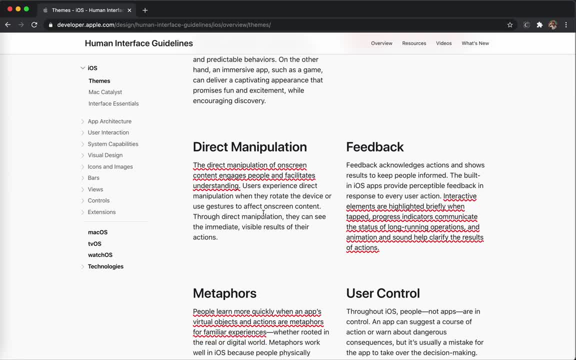 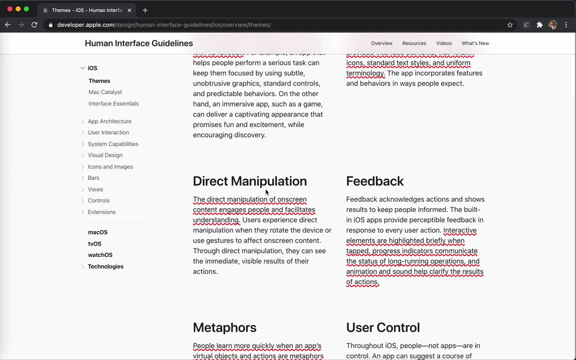 use gestures to effect on-screen con. I don't know direct to make it presentation this for iOS. I actually so if, uh, oh, yeah, I know what this is about. for this: desktop App applications. they actually are interacting with your apps through a keyboard or a mouse or a trackpad. 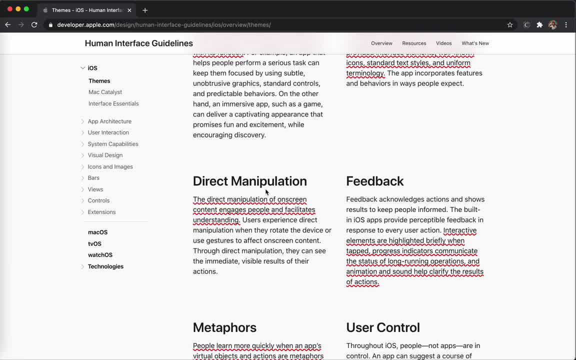 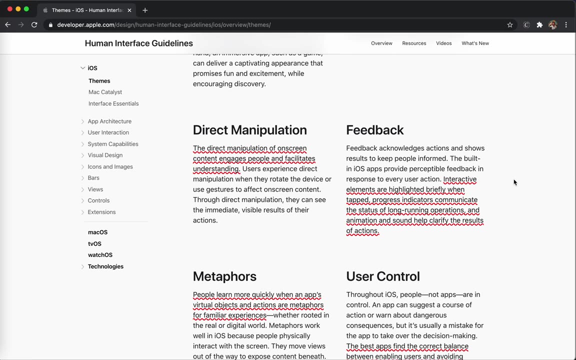 But on iOS devices they're using touchscreen, so they will touch your buttons, click your toggles directly, So that means direct manipulation. Feedback Interactive elements are highlighted briefly when tapped. Progress integrators communicate the status of long-running operations. This is also addressed by Google's guidelines of the idle process. 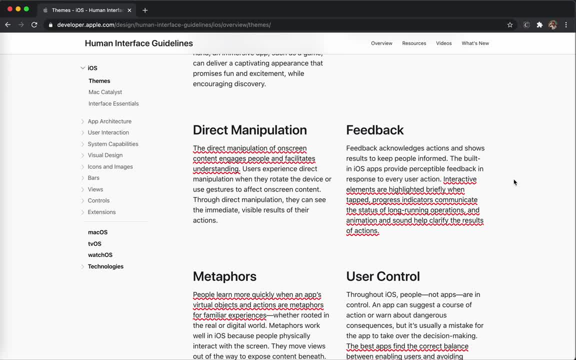 I mean the metrics by idle. It means that when a user interacts with your buttons or anything, you should give them the instant feedback. If it takes time, Use indicators. Loading indicators: Yeah, As the progress indicators here mean Yeah. 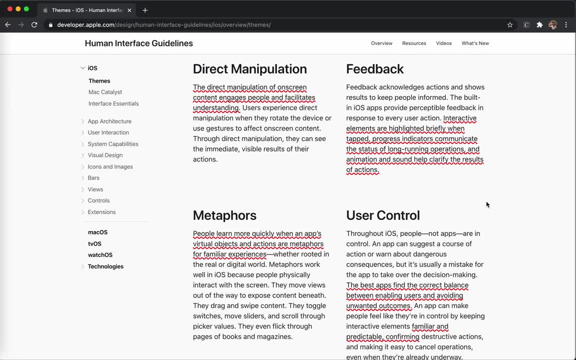 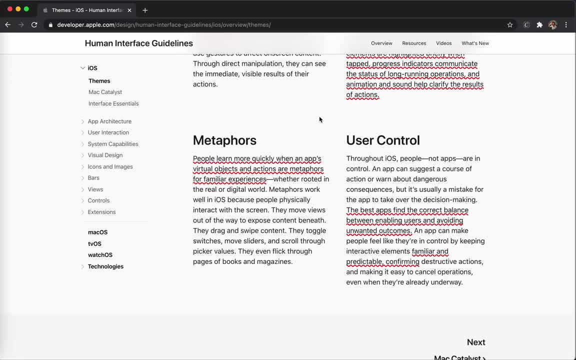 Don't let them think that your app is broken When they tap something, no response. That is not good. Okay, Metaphors: People learn more quickly when an app's virtual objects and actions are metaphors for familiar experiences. Yeah, 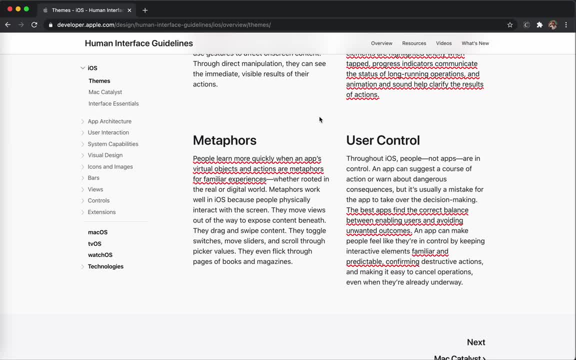 This is hard actually nowadays that people- actually there are not so many new, I would say interaction UI- creating it every day. They're using more like the controls from the old days. Yeah, They comply with the systems UIs, Like you see the sliders, the switches. 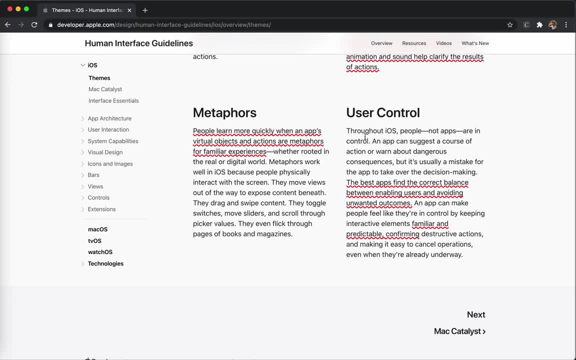 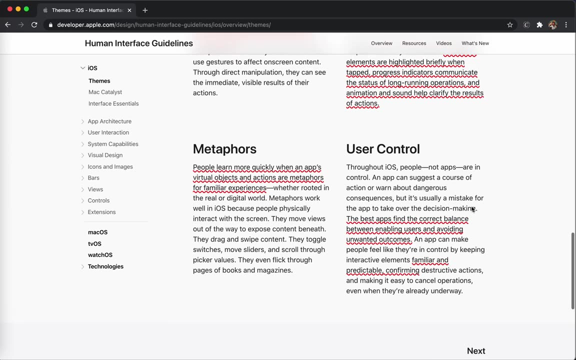 Yeah, Don't invent new ones. Okay, Use control, user control. The best apps find the correct balance between enabling users and avoid unwanted outcomes. It should be familiar, predictable and confirming. Yeah, As a web developers, we don't create new controls. 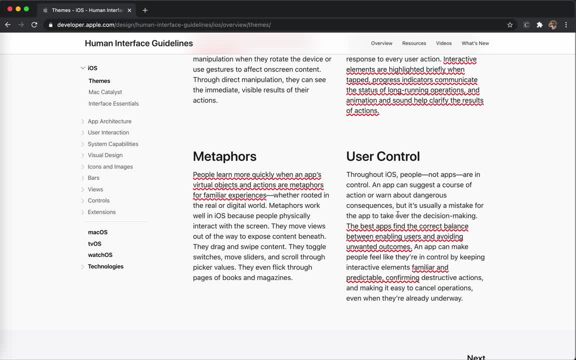 So we are using the native controls as the native apps, So that's not a big problems. The changes usually happens when the native apps creating something pretty cool and new, like the swipe to delete, delete, right. Well, that takes time. 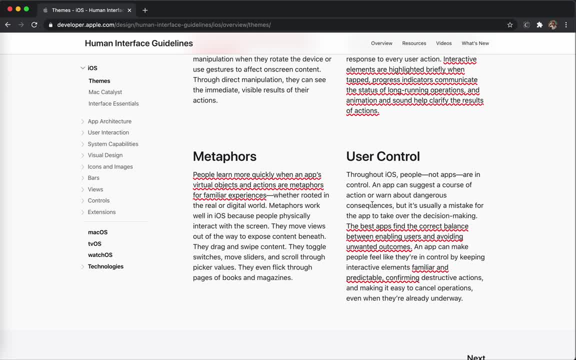 The users take some time to get used to that. And also the other one is the Twitter: swipe to refresh right, Swipe down, drag to refresh- Yeah, That's kind of metaphors and user controls- Yeah, Yeah, I think these two are similar. 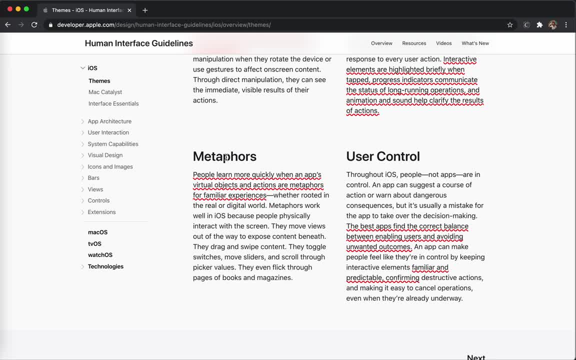 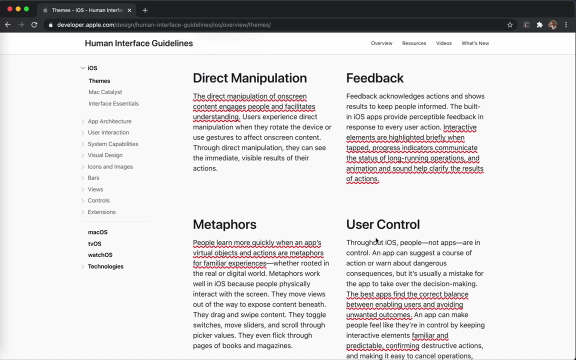 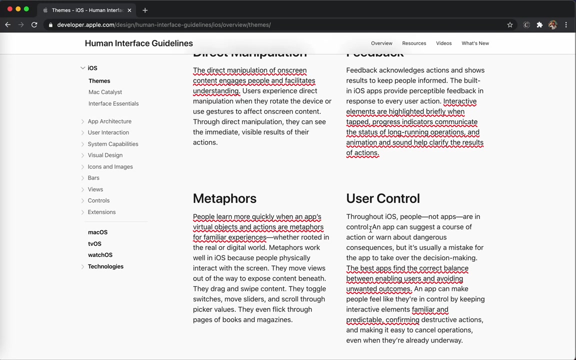 Metaphor, Anyway. so we don't create new user- how should I say new controls- without confidence, right? Unless you really need it And unless you're really sure that it helps create one, If not, use the old school. 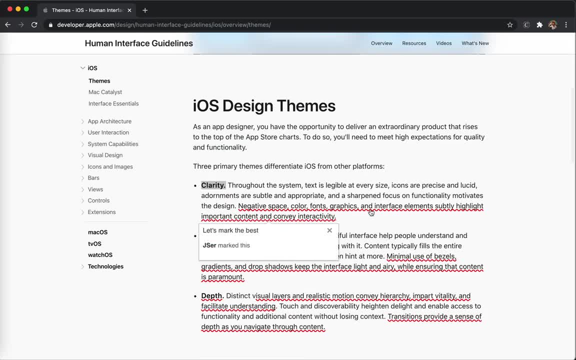 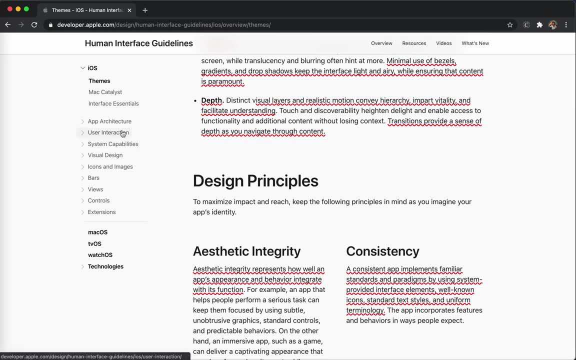 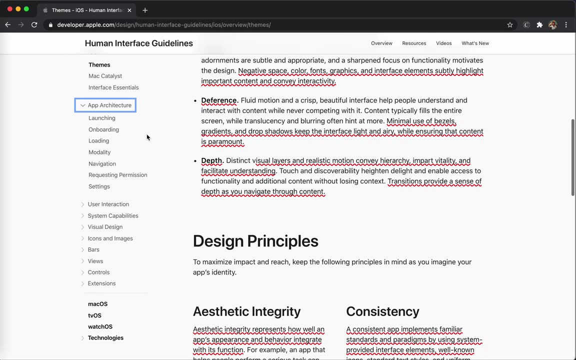 Controls. Okay, So this is the first one. I'm not sure this video helps you, but I'm going to continue creating these videos. I'm sorry If you don't help you. there are actually a lot of other topics, like the app architecture, launching, onboarding. 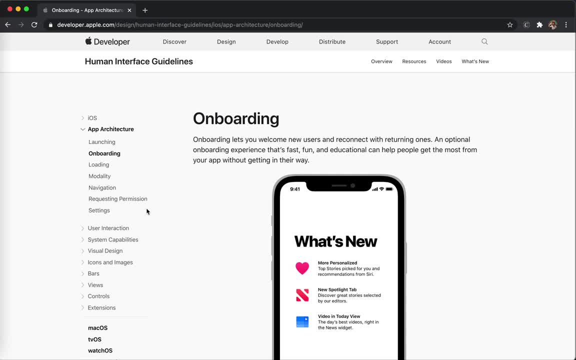 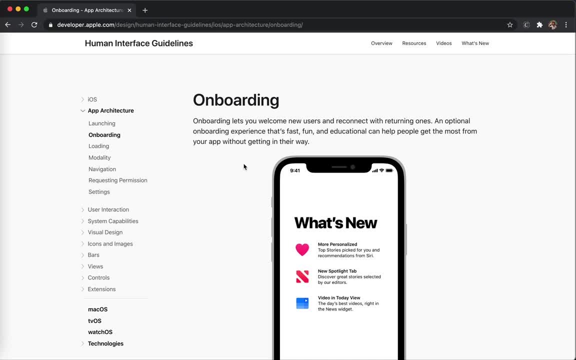 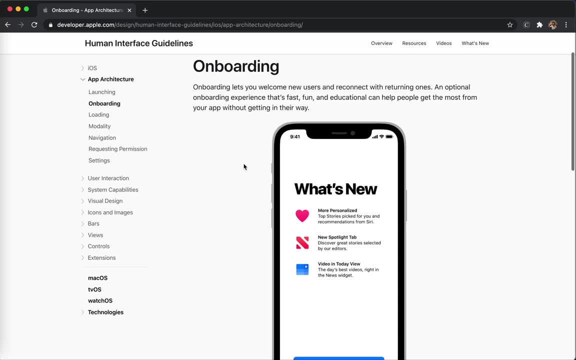 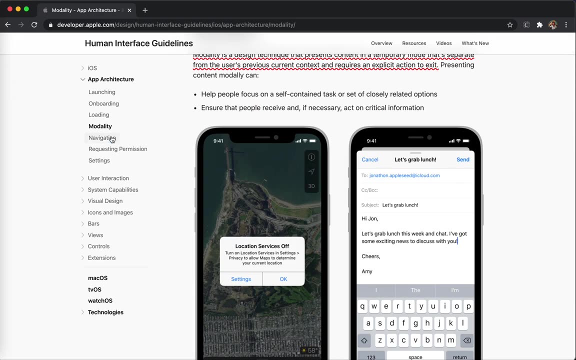 Yeah, We're currently like progressively creating web apps with the PWA stuff. Yeah, And loading also. we're using a lot of APIs. right Modality- This is commonly used- Navigation. This is actually the hurting point of web applications. 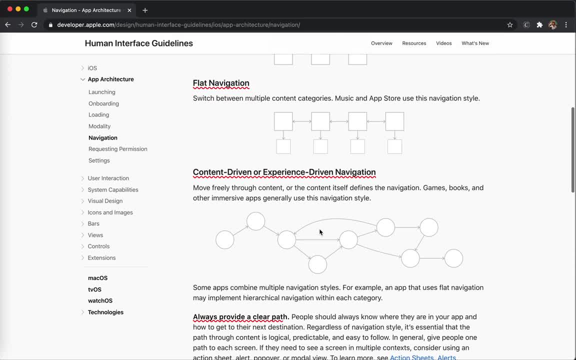 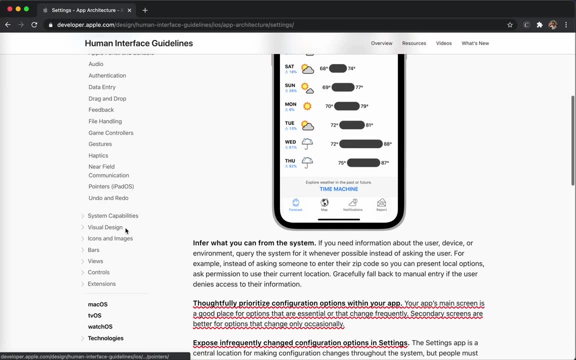 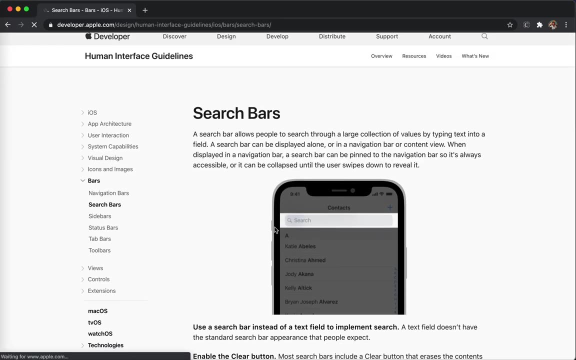 because the browsers have the native navigation buttons. It's not very cool actually- request permission settings, user interactions. Okay, let's jump through directly to the bars and views. You can see that navigation bars, the search bars, stuff like this. Okay, we'll cover this in the follow-up videos. 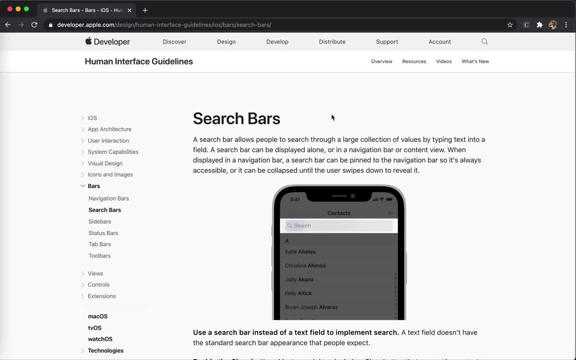 So stay tuned, See you next time. Bye-bye.